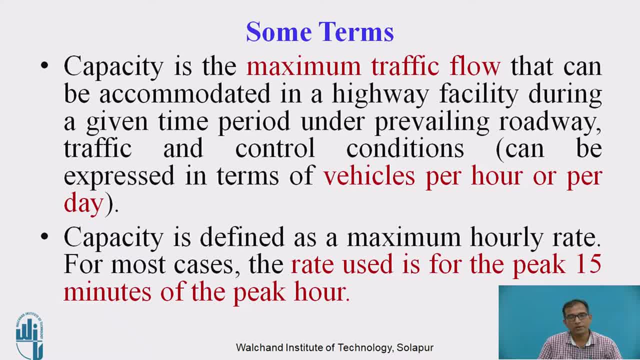 and how much it can take. take how much it can accommodate under the these conditions, prevailing roadway traffic and control conditions, keeping this is factors and measuring the capacity. so usually the capacity is defined for hourly rate or some cases, or most of the cases, the rate is used. 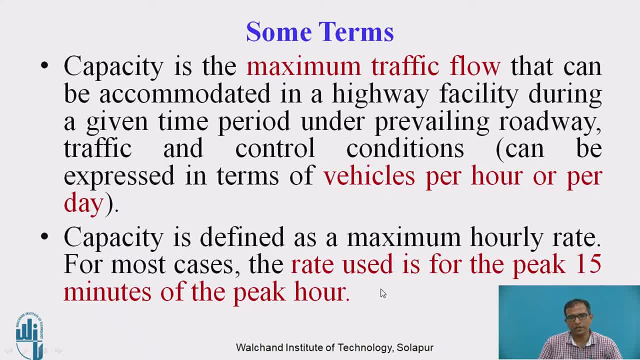 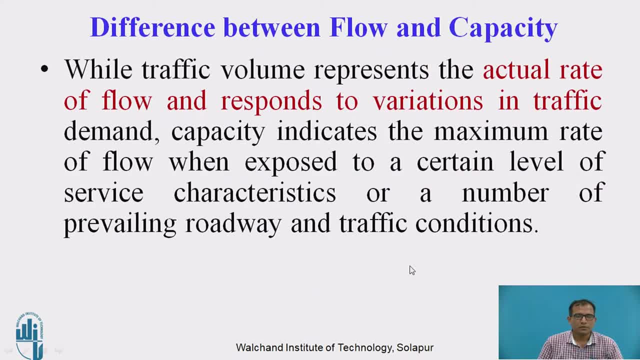 for the peak 15 minutes. for the peak hour. we can convert the peak hour 15 minutes into hourly rate also. so the difference between the flow and capacity. many of us may get confused. what is flow and what is capacity in this case? while traffic volume represents the actual rate of flow, 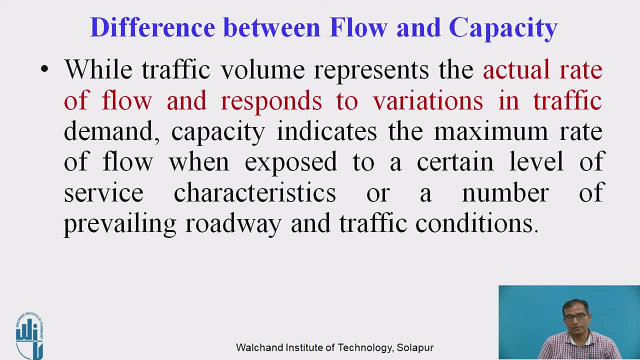 and response to the variations in traffic demand. so here the flow are, the volume. its going to response to the variations in traffic demand. it may be change the demand in the morning or change the demand in the evening also. so flow response: the variations in the traffic demand capacity indicates the maximum rate of flow it. its not talking about the what. 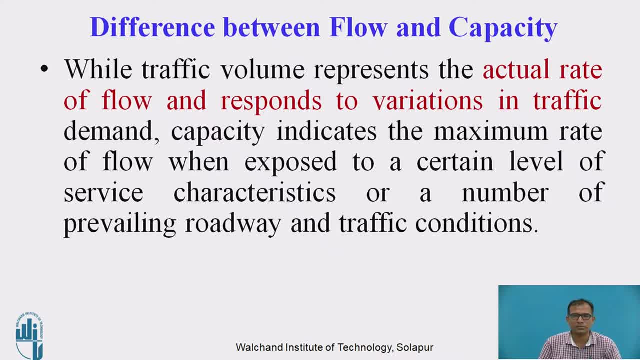 is the variations in the traffic. it tells about the numbers, the maximum rate of flow when exposed to a certain level of service, characteristics or number of prevailing roadway and traffic conditions. we will see that what is this prevailing roadway and traffic conditions? so what is the roadway conditions? it refers to the geometrical parameters of the road, such 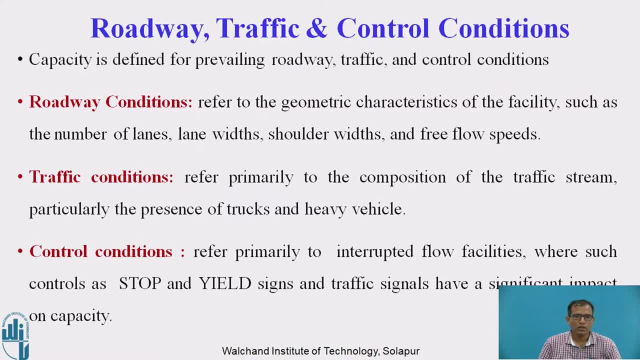 as the number of the road, not the distance, the traffic극 speed or the Gingerbread, i don't know. it will be difficult to understand. are we mushing VA Lukas seven solar station? this we can use. we can use this tool the small planes do this into. so this is a device get. 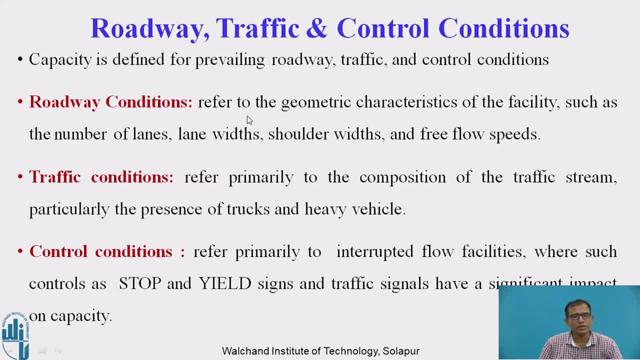 there are condition, all different equipment, one, some equipment ensuite, you will consider this with that, our계r resver, no so. activity terms, Control conditions, the number of the lanes, lane width, shoulder width and free flow speeds. So keeping these values and measuring the our capacity values, Traffic condition means without changing any. 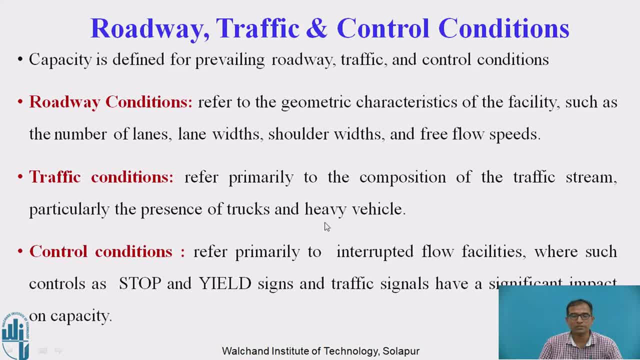 composition of the traffic stream, particularly the presence of trucks and heavy vehicle. and control conditions means primarily interrupted flow facilities where such control, like stop and yield signs, traffic signals, all these we have to keep it under conditions. under these conditions we have to measure the traffic parameters. 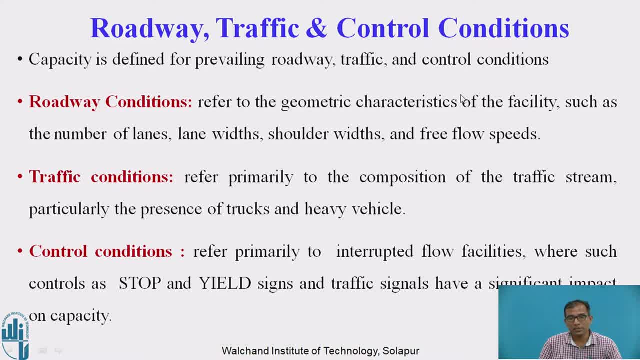 But prevailing this roadway traffic and control conditions is very difficult, but we, because every traffic stream is going to have interference of the traffic, other vehicles like trucks and heavy vehicles, or there is a change in the geometry or this- we have a stop or yield signs. 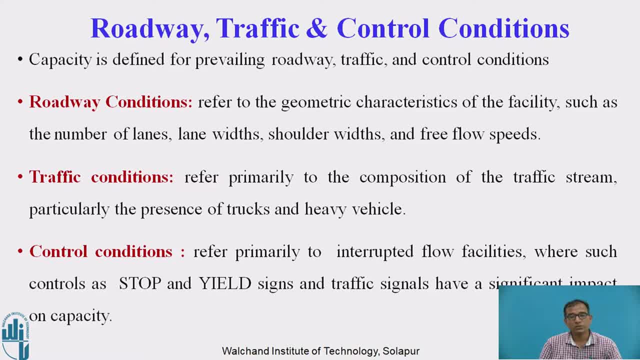 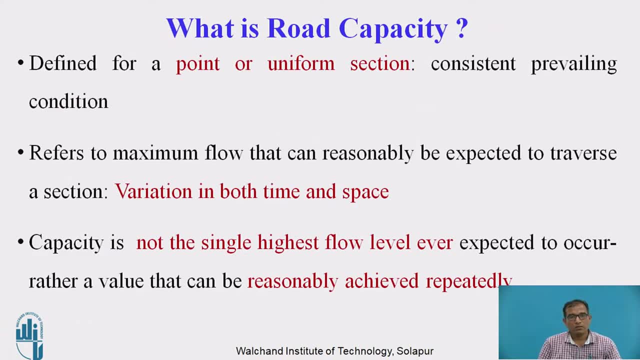 At the intersections, also due to the signals. so, keeping all these things, we have to measure the. what is the capacity of a road? It is, the capacity is defined at a particular point, or a particular stretch, or a particular segment, or a particular uniform section, consisting 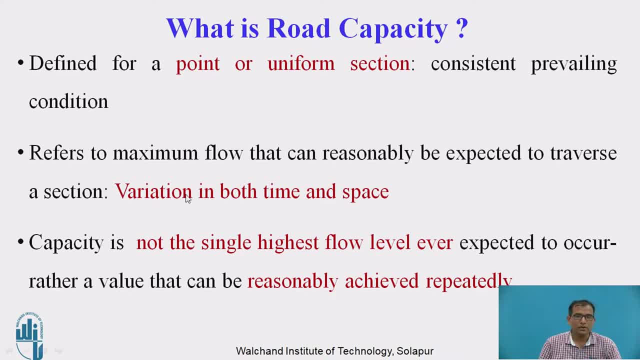 of prevailing conditions. So here the it refers to the maximum flow rate that can be reasonably expected to traverse a section. Even There can be variation in both time and space. The capacity will change according to the time and also space. capacity is not the single highest flow level ever expected to occur. 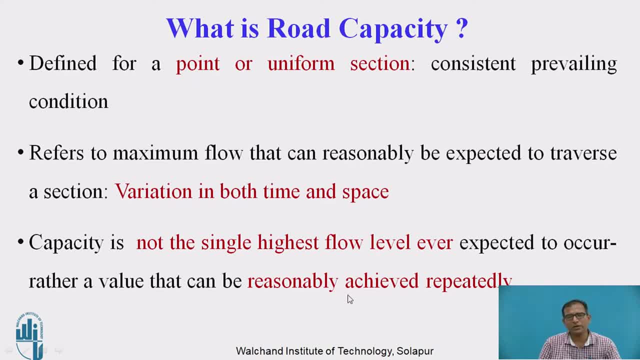 rather a value that can be reasonably achieved repeatedly. You can, you cannot say that it is a single value, highest value. Suppose the capacity is taken as something 2000 PCUs per day. so these 2000 PCUs per day can the vehicle, the, this capacity can be reached, this 2000 pcs per day, in that within the day 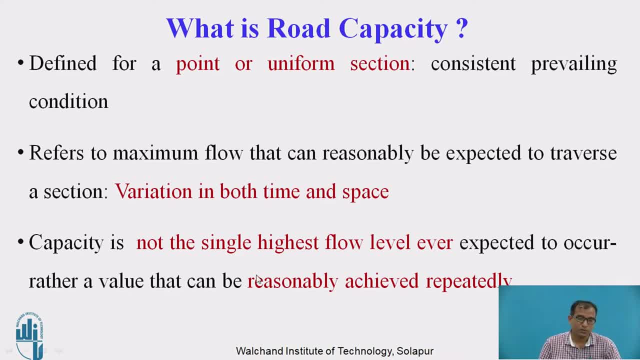 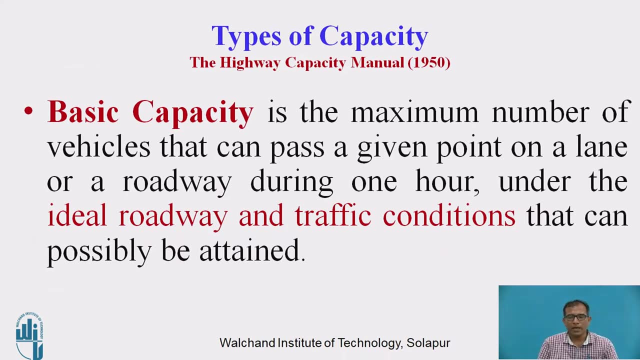 more than two times, more than three times also. so it is not the single highest value. it can be achieved repeatedly. that same value can be repeatedly achieved on that particular day. so basically, we have three types of the capacity. first one is a basic capacity. as per the highway capacity manual 1950, we have basic capacity. what is the basic capacity? 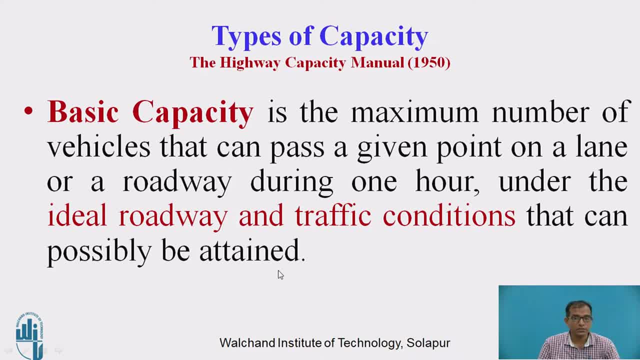 it is also called as a theoretical capacity. when you say theoretical, you are going to get it is a maximum capacity, maximum number of vehicles that can pass a given point on a lane or a roadway during one hour under the ideal roadway and traffic condition. this is very important ideal condition. just now we have seen that the traffic condition, the 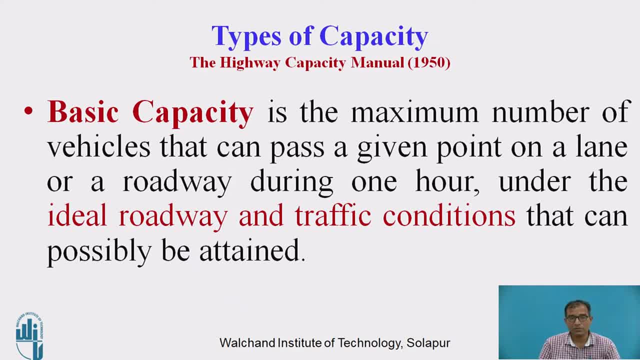 geometry condition: traffic stream characters. traffic stream characters characteristics- whether it becomes ideal roadway traffic where there is no hindrance from the other vehicle, there is no hindrance from the traffic signal. it is very seldomly. it is very, very difficult to get this ideal roadway condition. so if you are getting that, 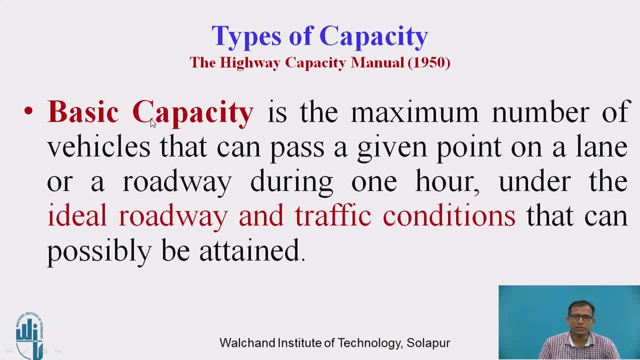 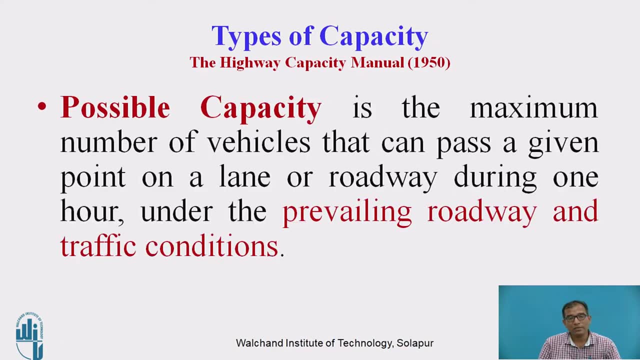 ideal roadway condition, then that capacity. you are measuring the number of vehicles flowing within peak 15 minute time. that capacity is called as a basic capacity but it is very difficult to get in the field. that is the reason we call this is the theoretical capacity. coming one next, a possible capacity. 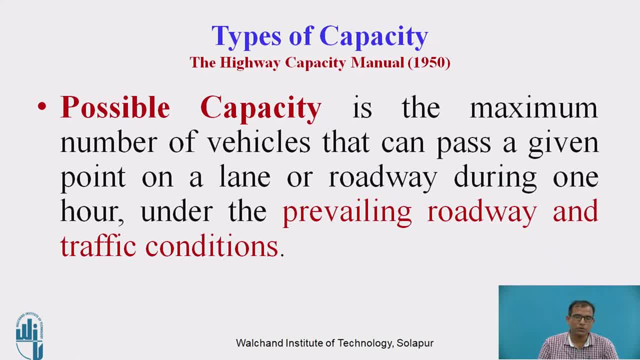 it is little bit lesser than the our theoretical capacity so it can be achieved. possible capacity is a maximum number of vehicle that can pass a given point or a lane, or you can take any stretch during one hour. you are measuring under prevailing roadway and traffic condition, so you are trying to come closer to the actual practical where you see that the prevailing roadways 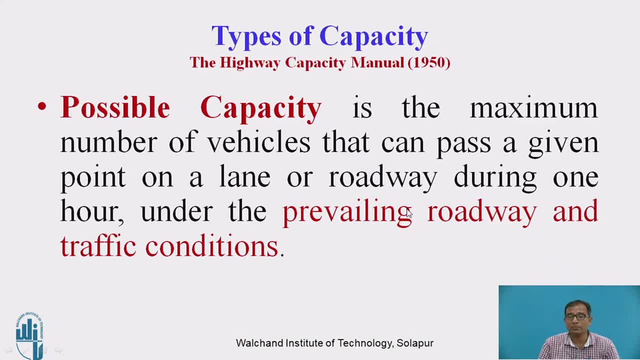 and traffic condition. again, it is very difficult to get prevailing roadways and traffic condition but when you come to the mixed traffic, there is a disturbance from another vehicle, there is a signal, there is a geometry hindrance, all the parameter we have to consider ideal. 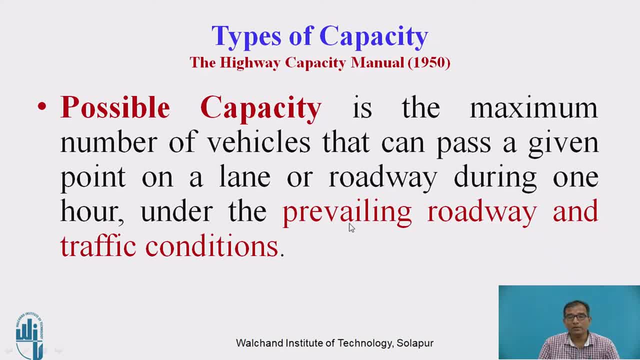 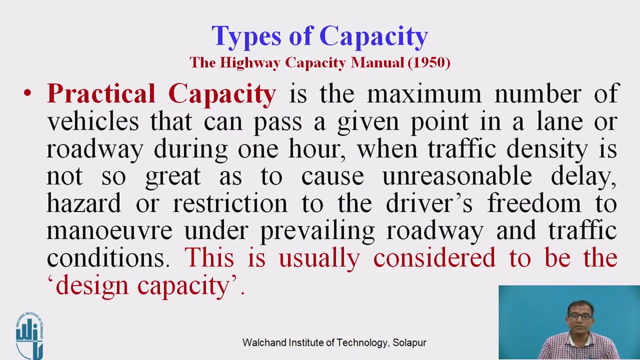 condition: ideal roadway and ideal condition: ideal roadway and traffic condition. it's difficult in the basic capacity- See here also possible capacity. also- it can be very, very difficult to get the both prevailing roadway and traffic conditions. So practical capacity is what neither we are not taking basic capacity or our possible. 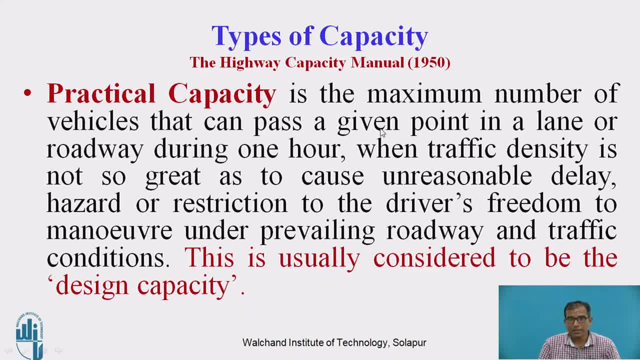 capacity. we are taking this practical capacity Here: the maximum number of vehicle that can pass a given point in a lane or a roadway during one hour. you can concentrate here when the density is here. we are talking about the, not talking about the. the other parameter we are talking- taking about the density- is. 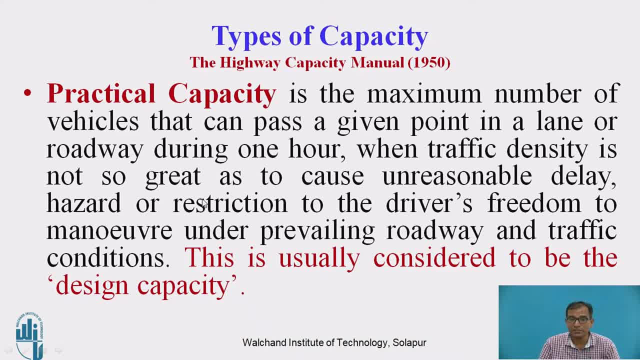 not so great. yes, there is a. the densities also exist and it is caused is unreasonable delay. also hazard or restriction to the driver freedom to maneuver under prevailing roadway and traffic condition. With the traffic stream you are measuring the capacity. that is what we call as a practical 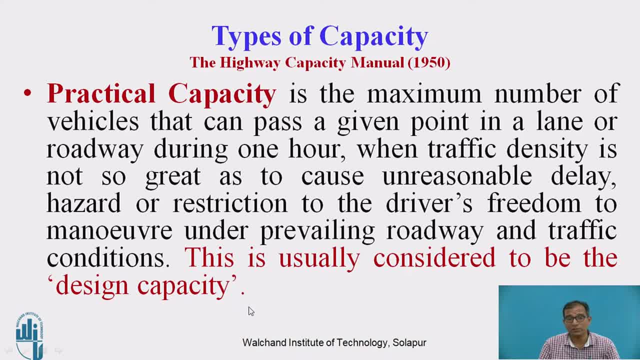 capacity. So this is usually considered to be the design capacity, because we are measuring the capacity with respect to the vehicle, With respect to the not theoretical, not possible, with respect to the our, the existing conditions of the road. that is the reason we called it is a practical capacity. 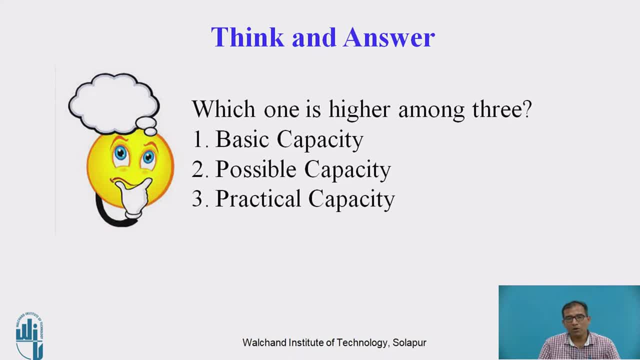 So you can think over here, you can think among this which one will be the higher, whether basic capacity, possible capacity or practical capacity, with explanation, I hope you are going to get the answer. in this reason, basic capacity is higher than possible capacity and possible capacity is higher than practical capacity. 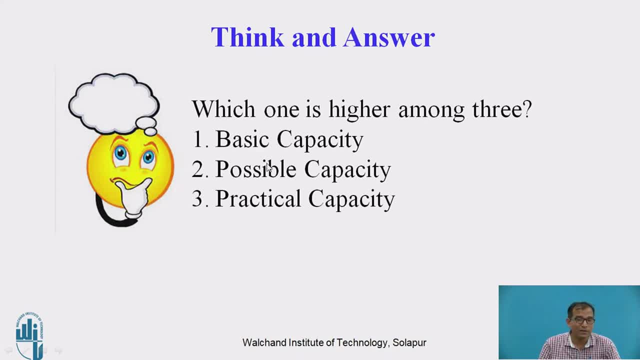 But in this, both the case, you are going to get ideal and prevailing condition. there is no disturbance from the traffic or signal. because of that, the number will be very high. that is very, very difficult to get that. sometime the possible capacity may become equal to the basic capacity. that is possible, but in this case basic capacity is more than possible. 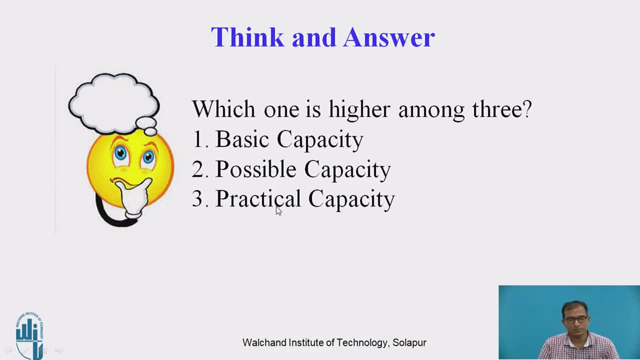 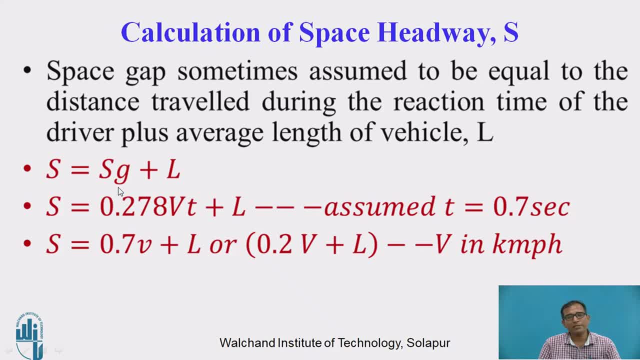 So calculation of this space headway It is sometimes it is taken as equal to the distance travelled during the reaction time of the driver plus the average length of the vehicle. If you take the, the average, the reaction time of the driver during the 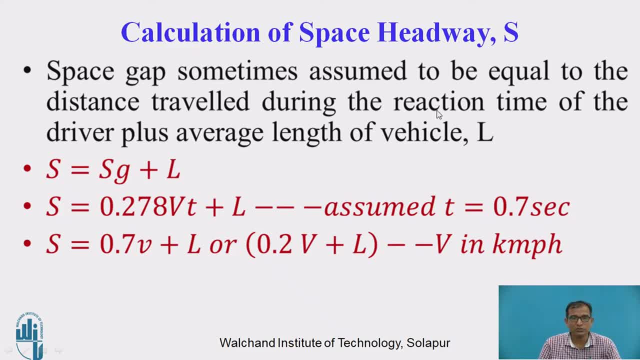 the perception distance. So that is what it is called as reaction time of the distance. Within that distance the driver will travel for some more distance. That is during the reaction time. So Sg is what the our reaction? the distance travel during the reaction time. 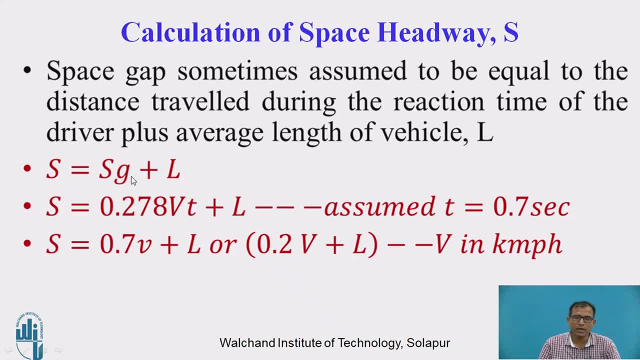 and L is the length of the vehicle. So this is already we have know when we are deriving the equation for stopping side distance in the highway geometry. there we know that the perception distance are reaction distance. it is a multiplication of the speed into reaction. 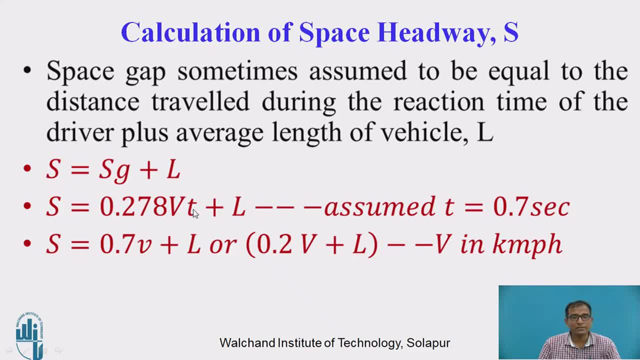 time. So here that small t indicates the reaction time. it is usually taken as 0.7 second, and if you want to convert that into kmph we have to multiply it 0.278 v into t. here v is in kmph. put the t value as 0.7 and simplify it further, it comes to 0.2 v plus L, that is. 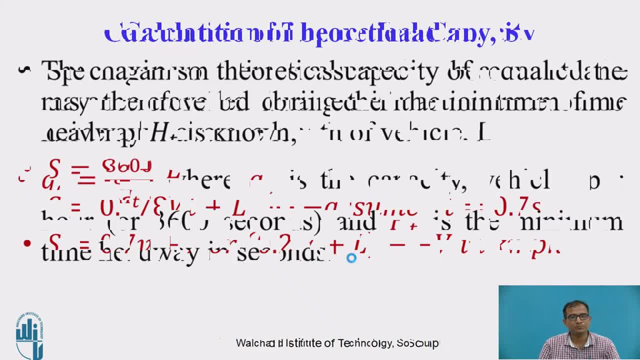 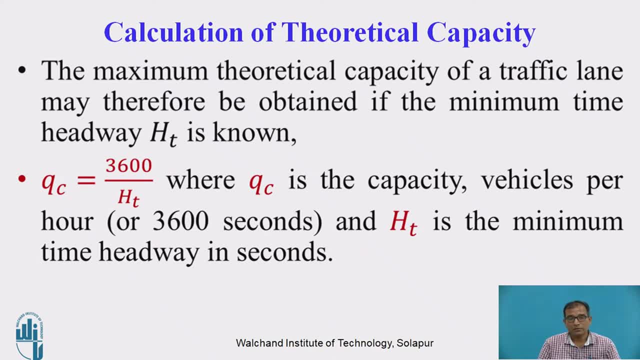 the space headway S where v in kmph. So when you have space headway, that is the equation, earlier equation- we are going to use it 1000 v upon S when we have headway in. So this is the equation: we are going to use it 1000 v upon S when we have headway. 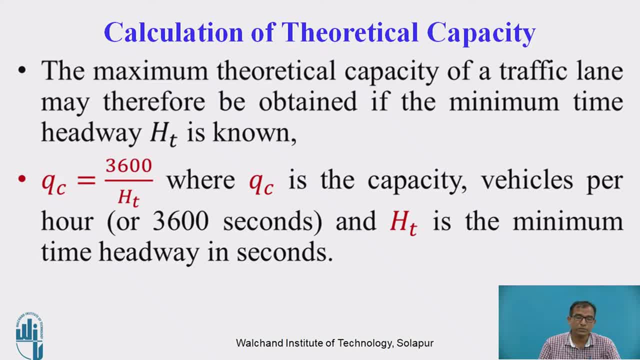 in time. we know that the headway is defined in two ways: space headway in distance and time headway in seconds. So when you have h t as the time there, you can define this maximum capacity or theoretical capacity, 3600 by h t in one hour. what is the total flow? 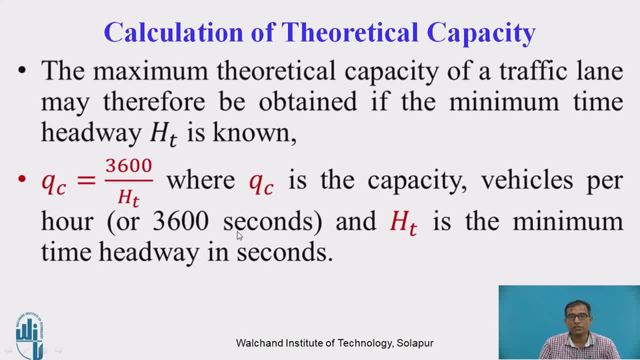 or capacity flow in one hour. that is the. it indicates 3600 seconds, where h, t is the minimum time. headway in second. So headway is what it is. This is the distance from the front of the vehicle to the another front of the vehicle. 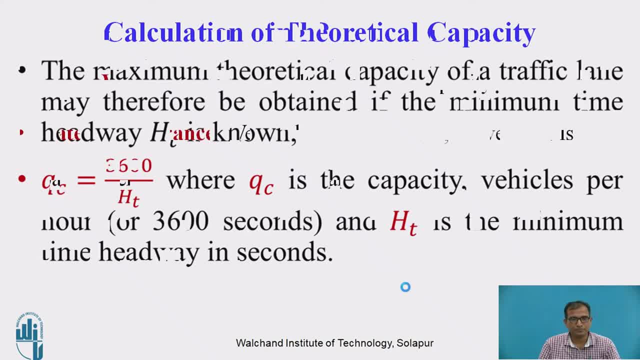 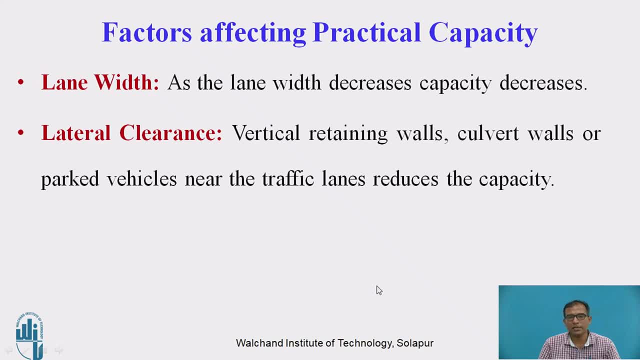 it is measured in distance as well as in time, So the factors are shown over here. it factors depends upon the, the lane width. as the lane width decreases, capacity decreases. lateral clearance about the different structures are coming in between. due to the some structure, your capacity may reduce And due to the narrow shoulder S capacity. 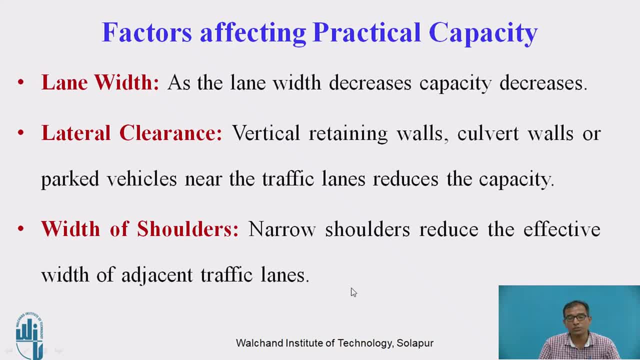 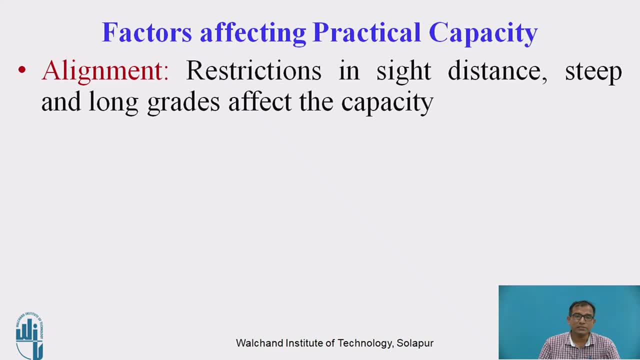 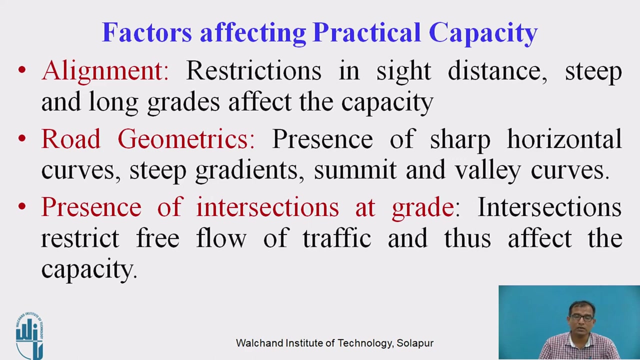 will reduce because some time during the emergency we may use the shoulder to increase the capacity. Alignment restrictions in the side distance, steep and long grid affect the capacity. it reduces the capacity. a steep gradients are sharp curves that may reduce the capacity. presence of intersections at grade S the more the intersections are coming in the highway.